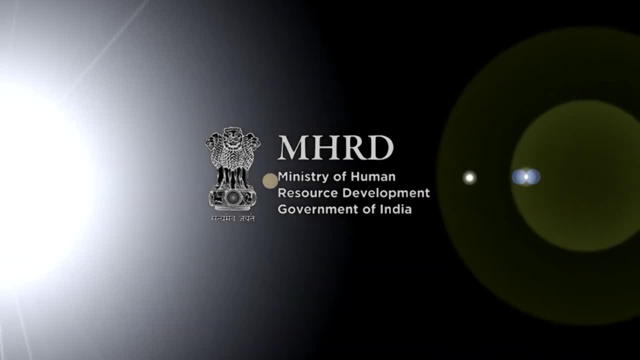 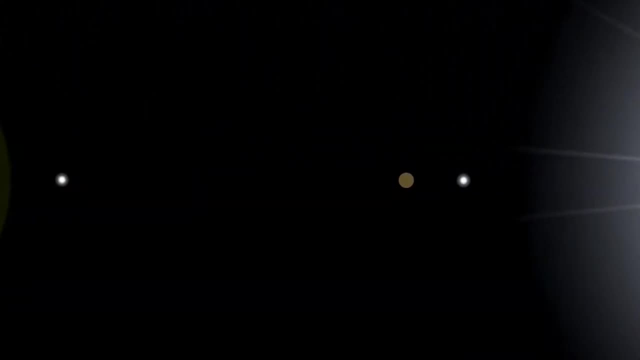 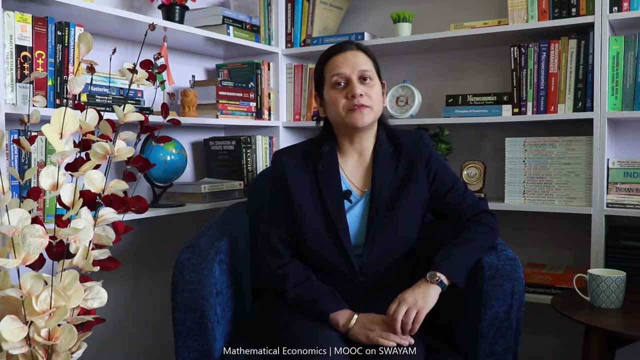 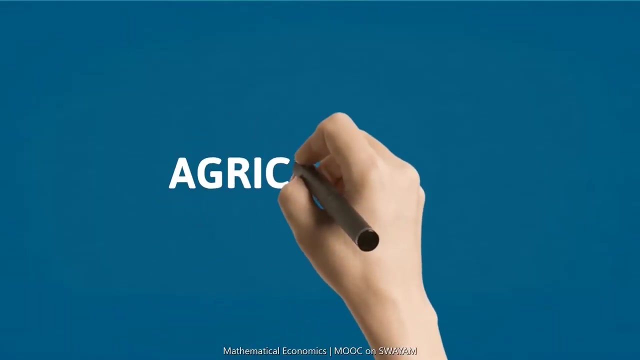 In the previous video, you were introduced to a new technique called Linear Programming. Are you curious to know more about this technique? You will be surprised to see the applications of Linear Programming in various fields. This video will show you the various applications of Linear Programming. Check this out. 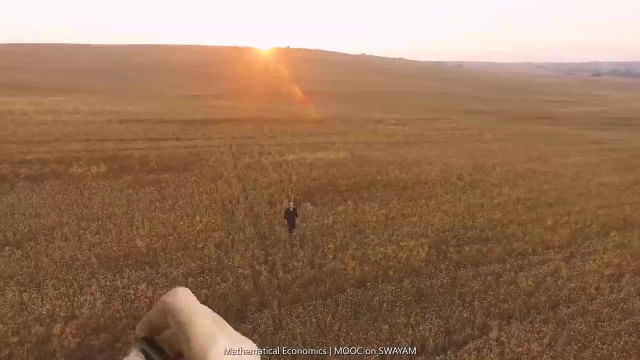 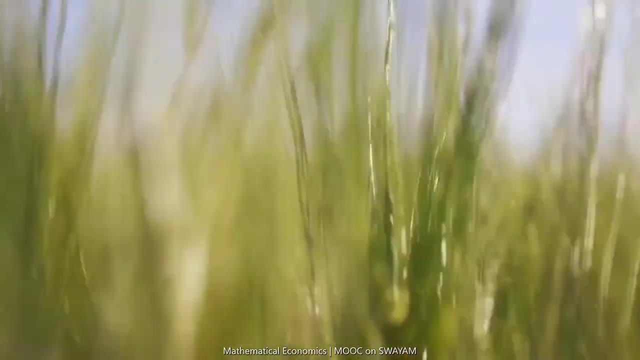 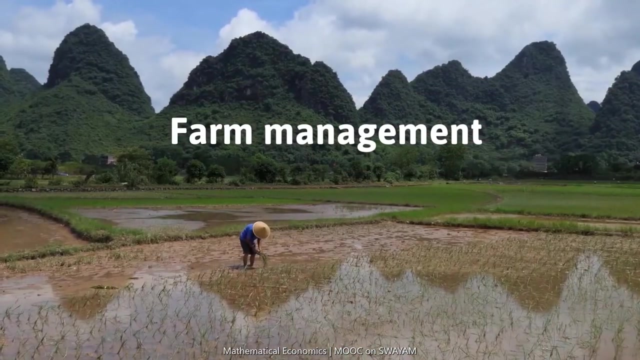 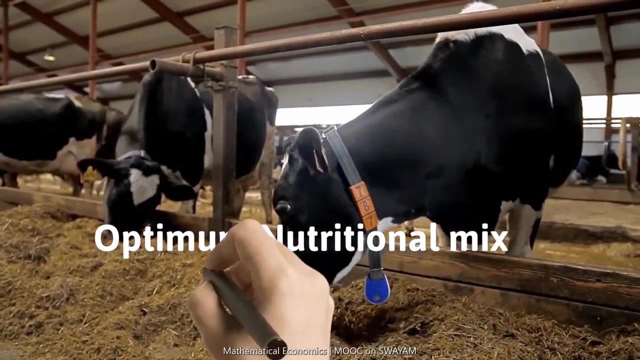 Agriculture is the backbone of the Indian economy. Have you ever wondered how agricultural lands are allocated to various crops for higher yield so it meets the need of the burgeoning population? How are farms managed within environmental, legal and social-cultural constraints? What is the best nutritional mix for feeding? 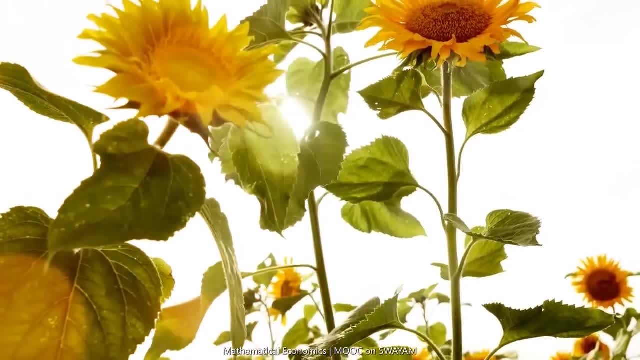 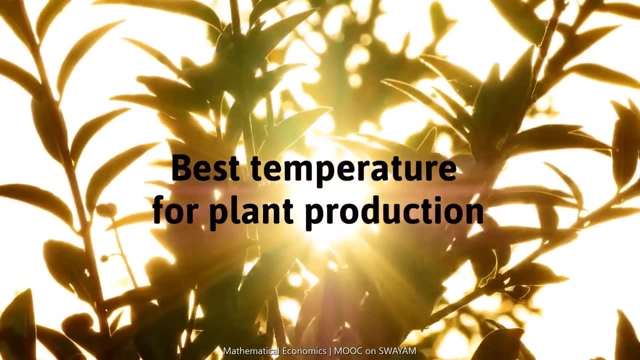 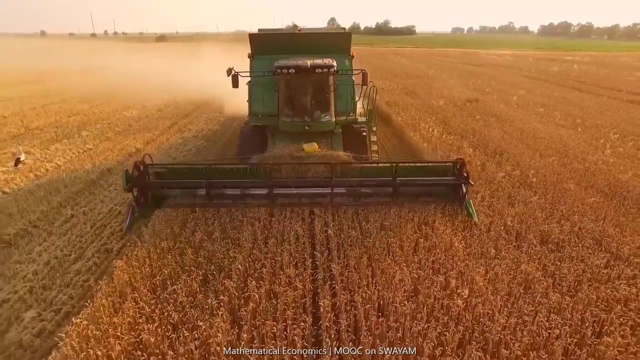 the livestock. It is known that high temperature affects production. How is the best temperature selected for plant production for maximizing the profit? Decision making in agriculture is based on scientific planning, and linear programming play a very important role. Thank you for watching this video. 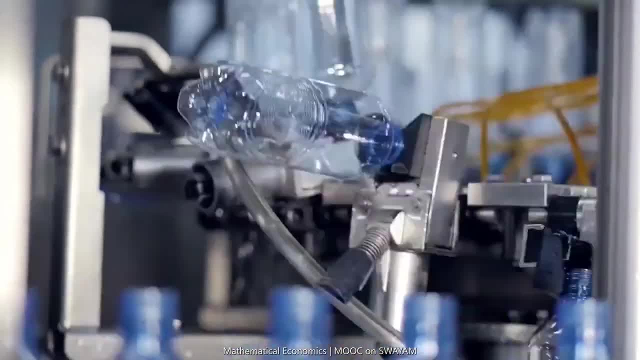 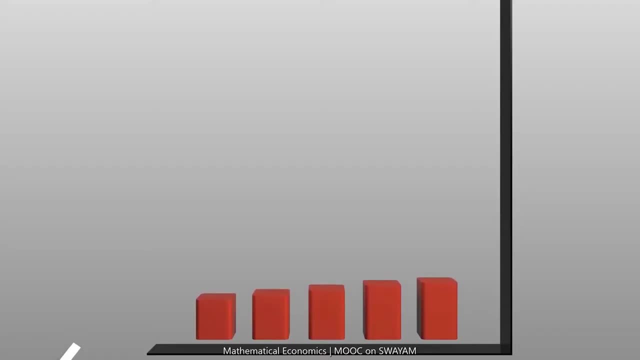 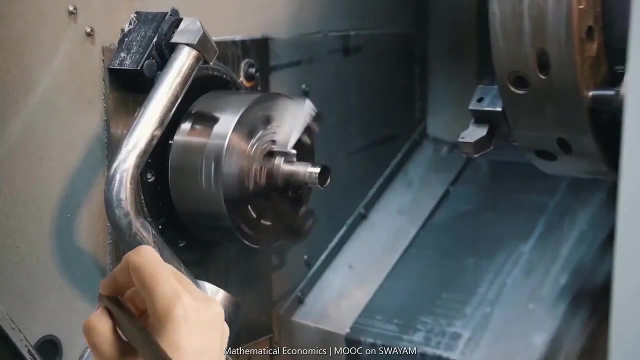 What is the main objective of manufacturing industries? You are right, It is to maximize profit or return. Apart from maximizing profit, there are other problems such as optimization of production scheduling, ie allocation of resources, events, processes to produce goods, optimization of product mix problem and the 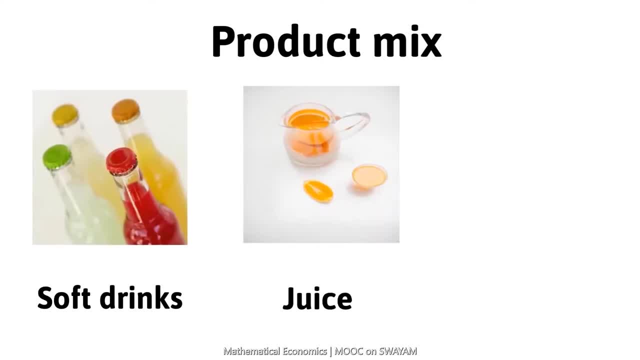 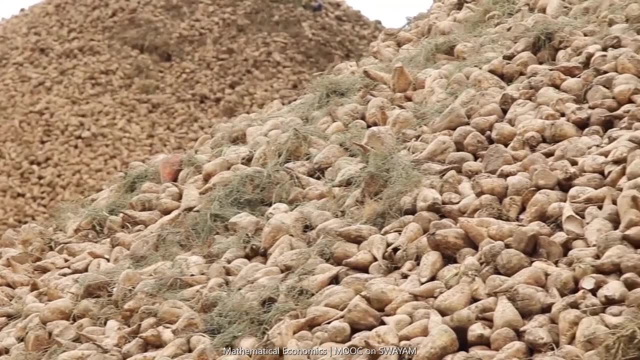 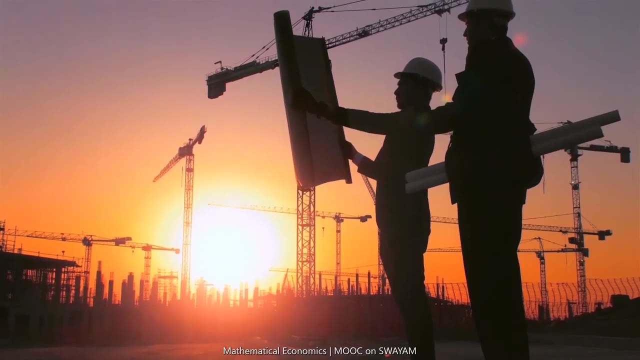 cost of production. That is how to get the best from different product lines of a company And optimal use of raw materials. For example, Material efficiency in construction can be less expensive and energy intensive. Material efficiency includes reducing energy demand, reducing harmful emissions and other. 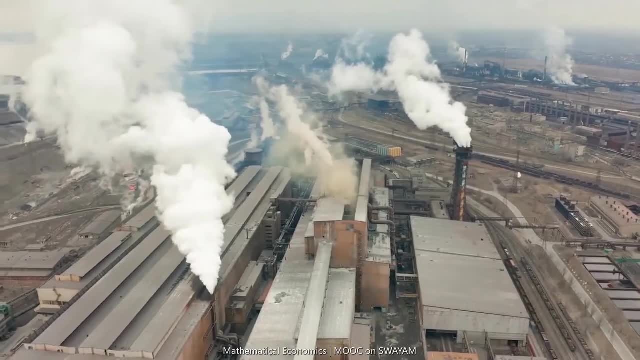 environmental impacts. In addition, the production process of raw materials is made up of materials which are usually used every day for production. The cost of staples is also reduced. Minimizing material consumption during production may help to reduce the cost of raw materials. 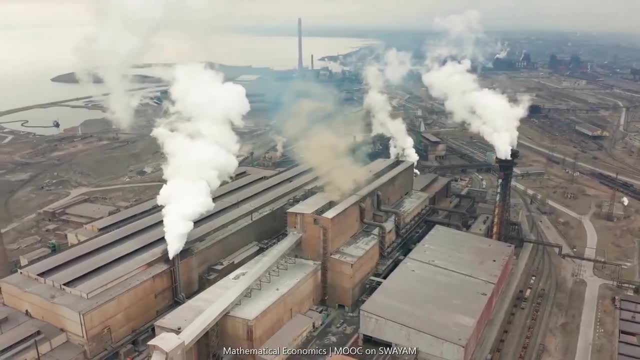 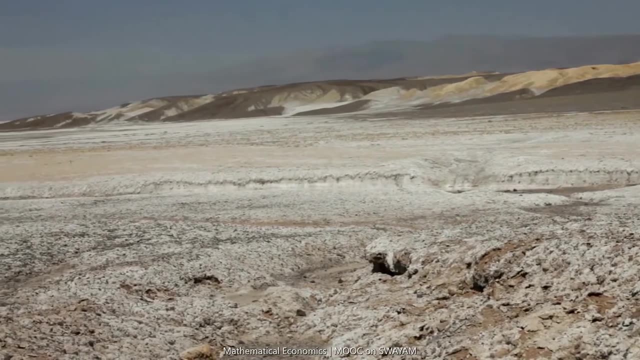 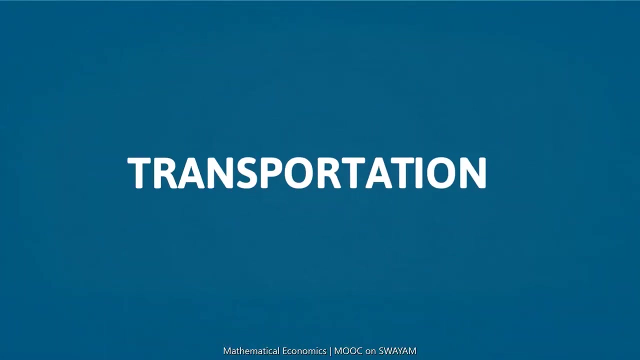 So that is our important point. Now. please comment. Do you have any other questions that you wish to discuss in the next? impacts of industry and increasing national resource security? all these problems can be solved by using the concept of linear programming. transportation means moving from one place to. 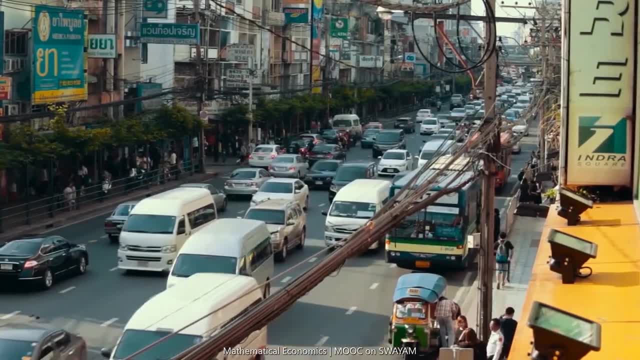 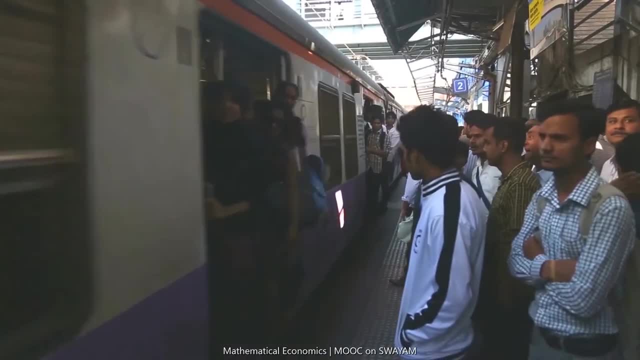 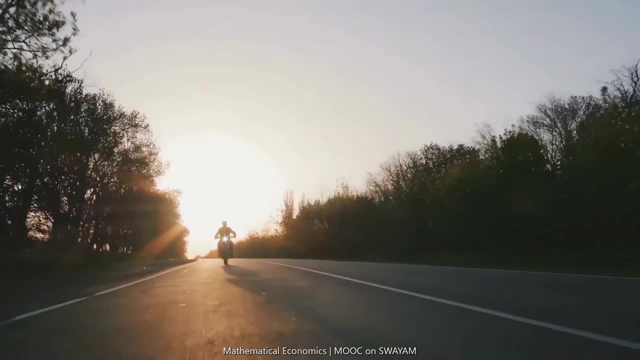 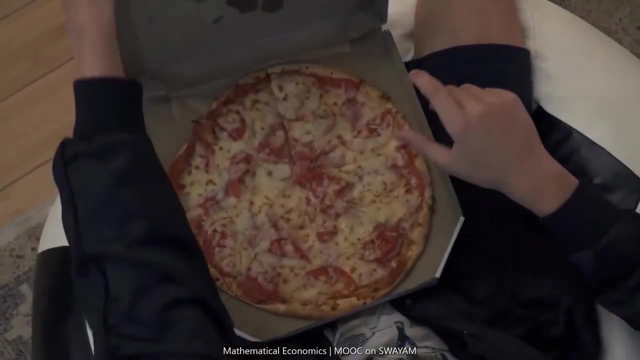 another. the transportation problem is based on the supply and demand of commodities or people from different sources to different destinations. for example, what is the shortest route that a pizza delivery boy should take so as to minimize the cost and time taken to deliver the pizza to a particular destination and return to his workplace? 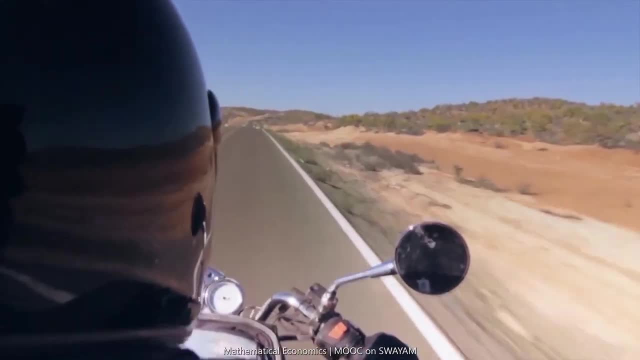 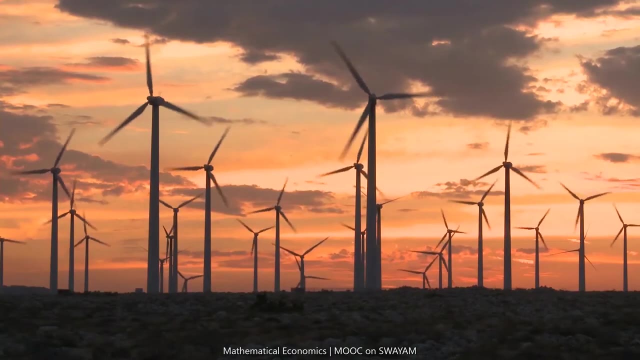 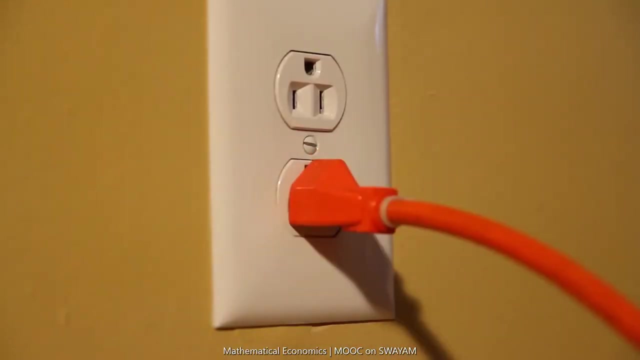 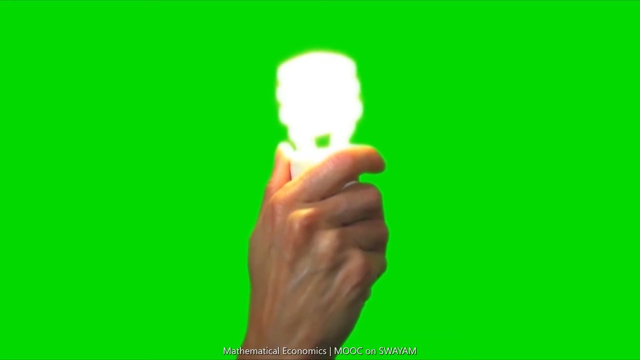 linear programming may be used to reduce the transportation cost. linear programming may be used to reduce the transportation cost. linear programming may be used to reduce the transportation cost. linear programming may be used to maximize energy savings or reduce energy consumption of households. you must have heard about led bulbs. led means light emitting diode. these are the most energy. 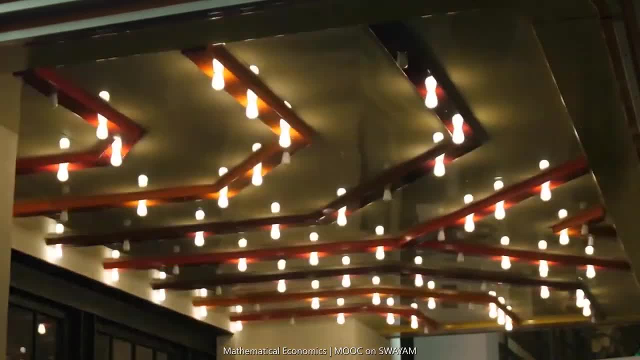 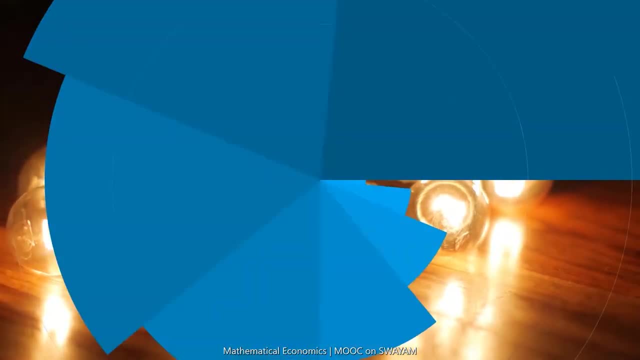 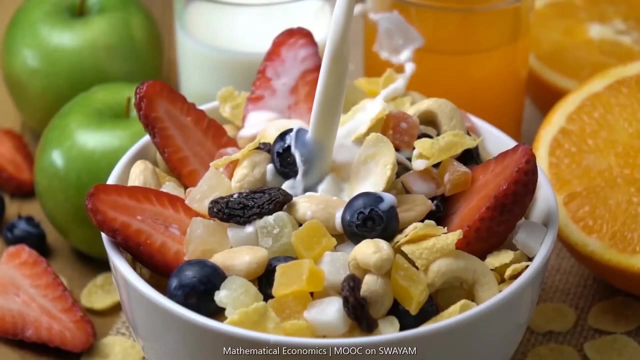 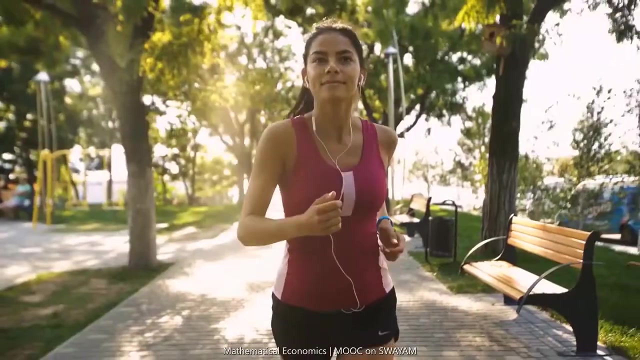 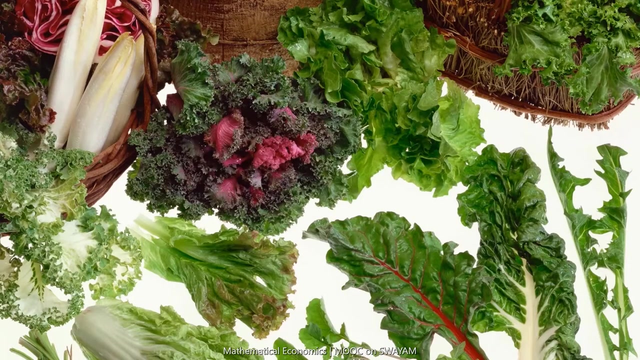 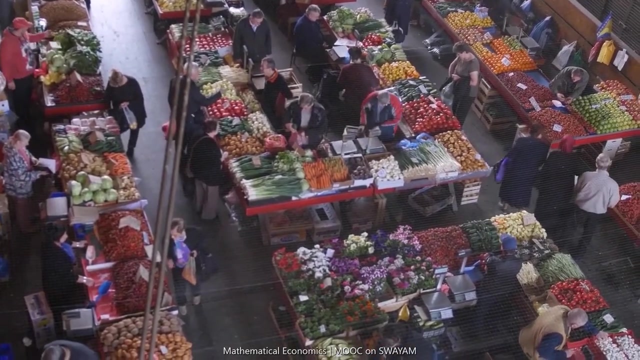 efficient lighting option. led bulbs use 75 percent less electricity than the ordinary light bulbs and policy can be eliminated when you use 15. it can make such a safety commitment. a balanced diet is a diet that gives the body the minimum nutrients to function properly. green leafy vegetables and other raw vegetables and fruits contribute to a healthy diet. certain food in the market are very costly, but a healthy diet includes whole grains or whole gliobes is what they will do to help the body, and with home food it is easy for alcoholics to be advised, but health food and water will be poor, as they provide potent results in terms of nutrition. 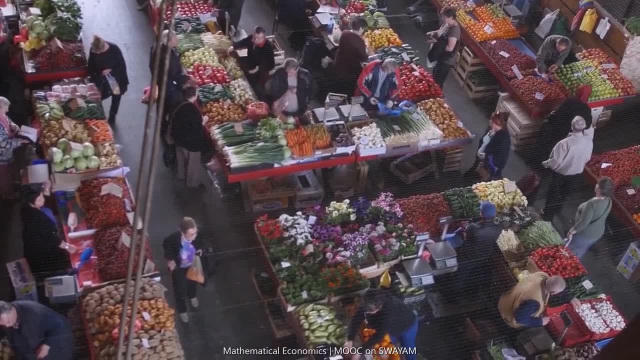 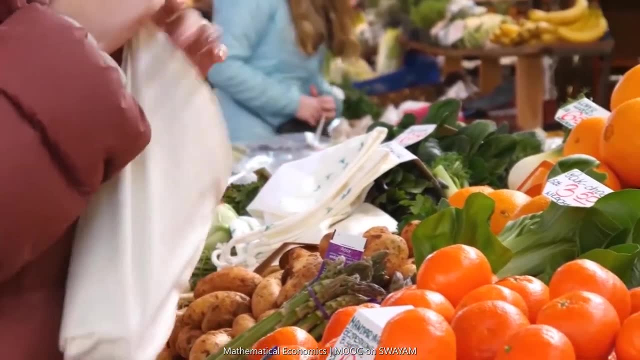 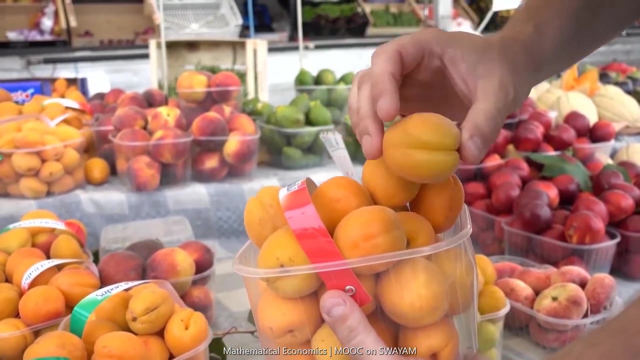 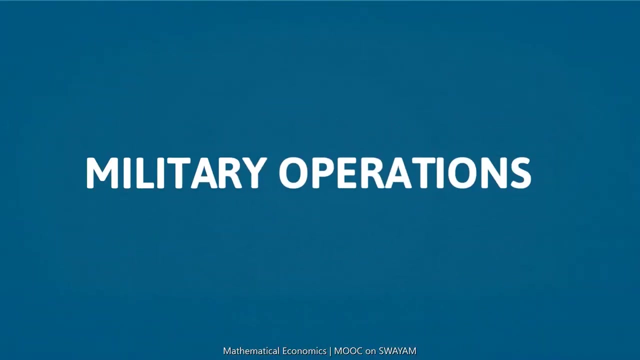 diet is also essential, so what quantity of each food should be purchased so that the nutritional requirements for the body is fulfilled at a minimum cost? solutions to such diet related problems use the technique of linear programming. we have seen in the previous video that the use of linear programming started. 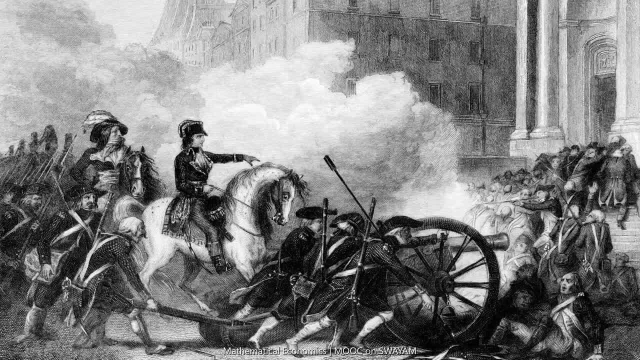 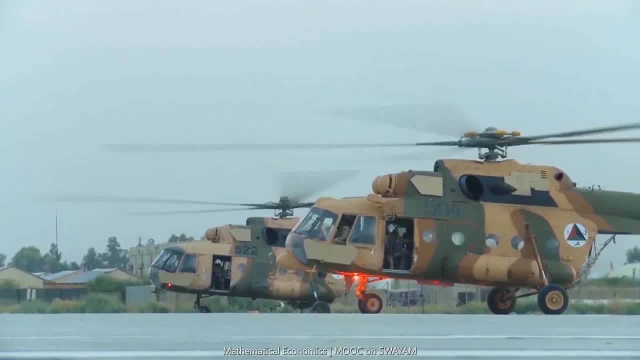 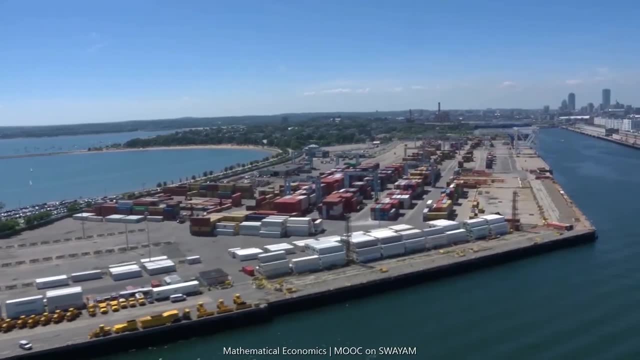 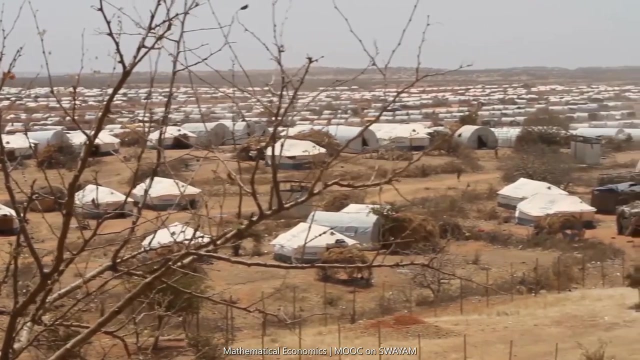 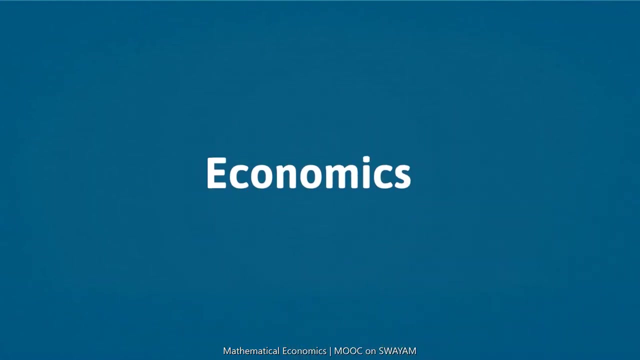 during the Second World War to minimize the losses brought about by the enemy. a number of military problems, such as army logistics, wartime patient evacuation, cargo distribution and regulating other military operations during a crisis, can be solved using the technique of linear programming. you economic problems such as maximizing profit, revenue, sales, minimizing the cost. 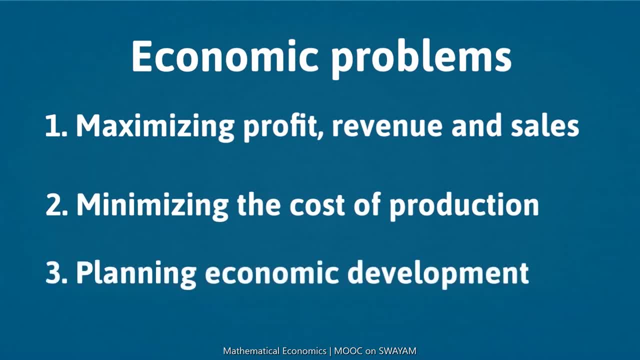 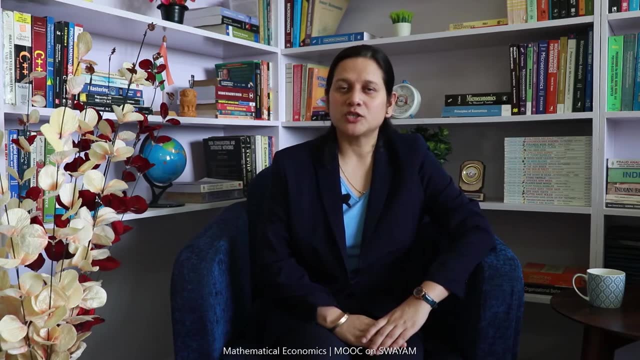 of production and planning economic development use linear programming models. a couple of these problems will be discussed in detail later this week. so we have entered into a new world of programming. optimization is the main objective of different professions such as business, finance, engineering, architecture, computer programming and research. in the next few videos you will explore the linear programming in detail. 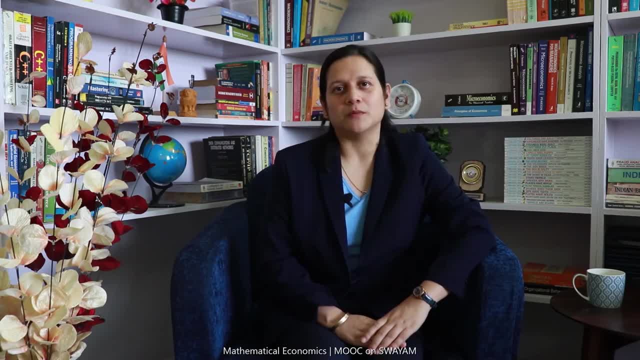 and create programs to solve some economic problems. Ocean Animals. A little over 70% of our Earth is covered by oceans. There are five oceans: Pacific, Atlantic, Indian, Southern and Arctic. Within our oceans live thousands of plants and animals. Many of them haven't even been discovered yet. 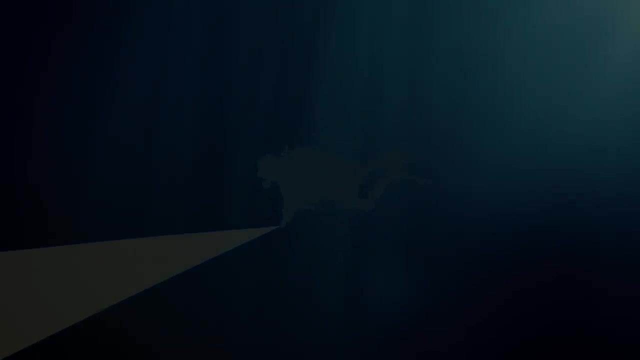 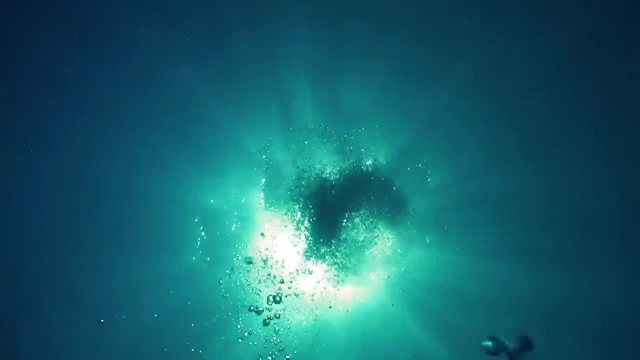 The deepest parts of the ocean have little or no plant life. That's because the energy from the sun cannot reach deep into the ocean and plants need sunlight to survive. However, there is an abundance of plant life or seaweed wherever the sun can reach. Seaweed is the name for many different types of algae and plants that grow in the ocean. Seaweed is a type of algae that floats on the surface of the water. Another type of algae in our oceans is called phytoplankton. 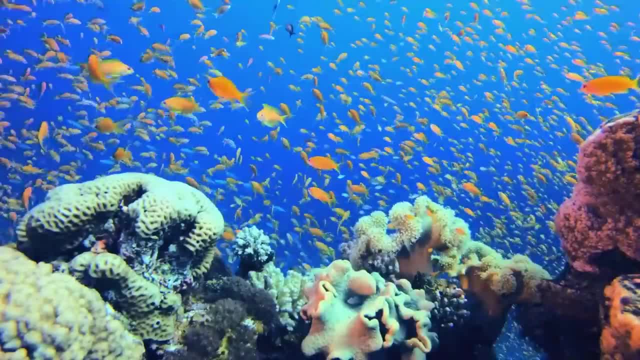 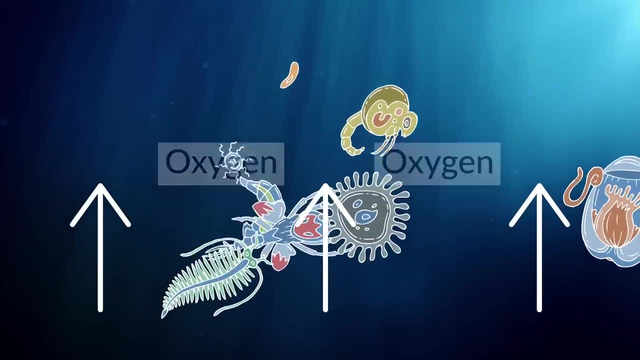 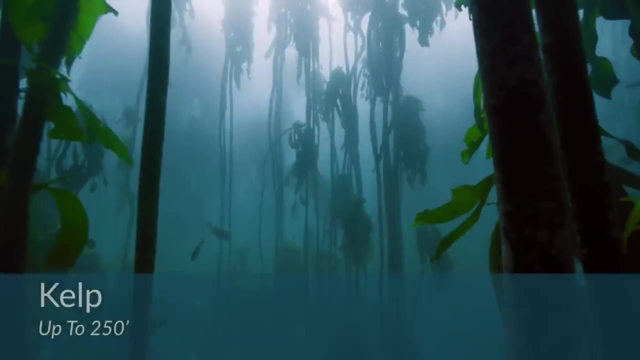 It is extremely tiny but very important. Living organisms depend on phytoplankton for food. This plant gives off more oxygen than any other plant on Earth. The largest ocean plant in the world is called kelp. Kelp grows very quickly and can reach up to 250 feet tall. 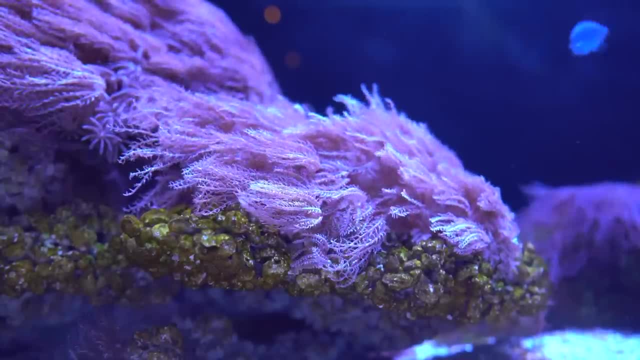 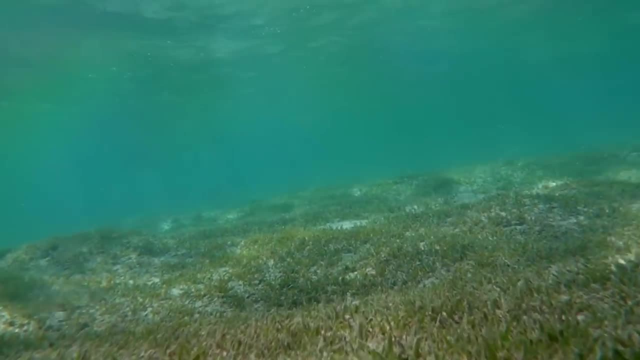 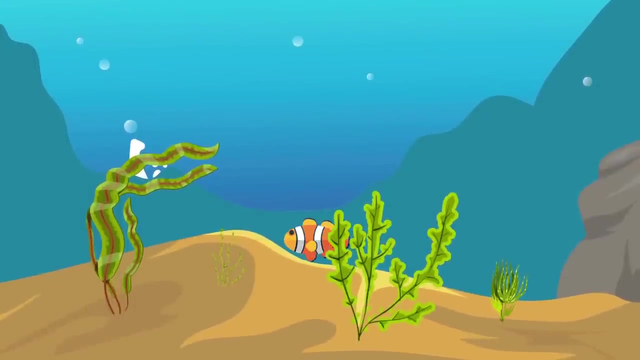 It is usually brown, but some kelp can be very small. It can be very colorful. Seagrass is another type of plant. It grows in the shallow water of our oceans. It has roots and flowers. There are numerous plants in the ocean that are similar to algae and seaweed.